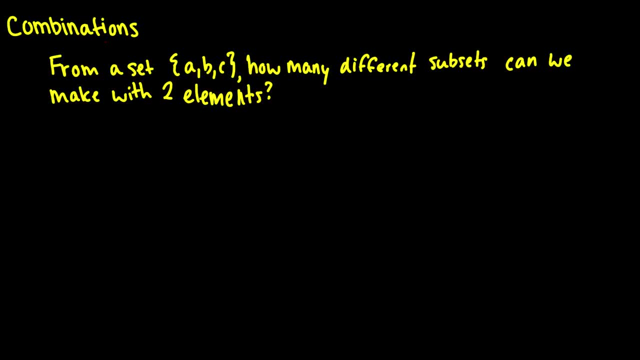 and two ways to pick. the second one because if the order is switched it doesn't necessarily make a difference. For instance, in a permutation the order ABC and ACB are different. so this is two, But in a combination, If we have ABC it is going to be equal to ACB. They are the same thing. So now that 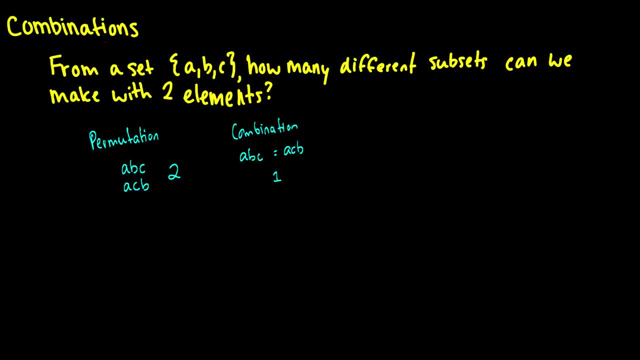 we've dealt with the differences here. how many different ways can we make a subset with just two of the elements? Well, let's just list them all, So we can have A and B together, we can have A and C together. we can have B and C together. 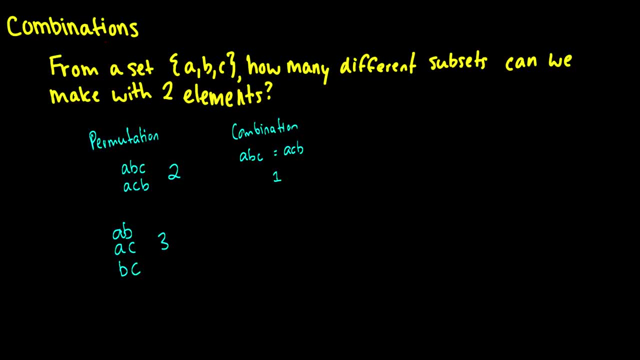 So these are three different ways. Now you're saying: well, what about BA, what about CA and what about CB? Well, these map to ones we've already done, so we simply don't count these. So what we say is that there's three different combinations we can make. 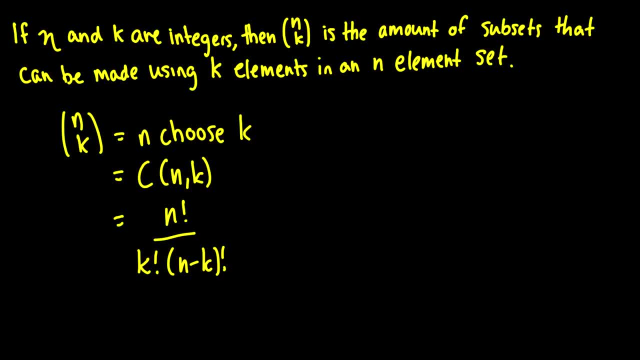 So here's a nice formula for it. If we have two numbers, N and K, then we say that N choose K is the amount of subsets that can be made using K elements in an N element set. So this is written as N choose K. Sometimes you see it as a capital C with N bracket or N comma. 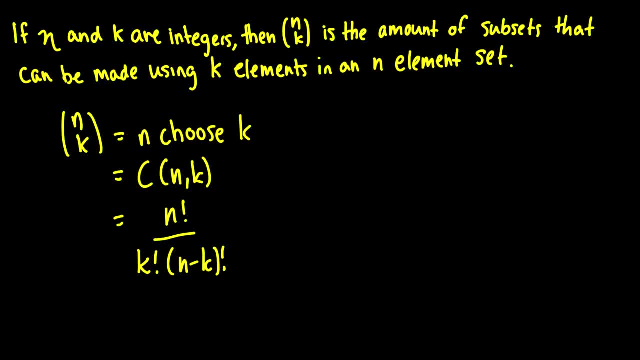 K, just like permutations, And we see the formula here: is N factorial over K factorial, times N minus K factorial, which you'll see is actually just the permutation function divided by K factorial, which is the number of elements we're making. So in the previous 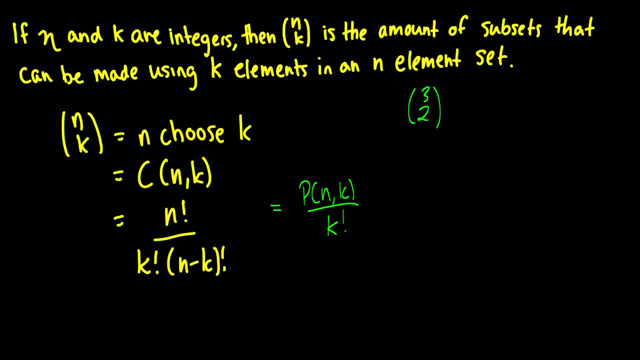 example, you saw three choose two, because we wanted two element combinations out of a three total set. So with this formula, this is going to be three factorial over K factorial is going to be two factorial and N minus K is going to be one factorial, which is going 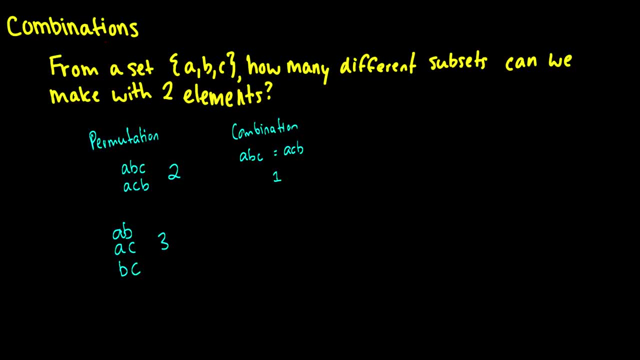 So these are three different ways. Now you're saying: well, what about BA, what about CA and what about CB? Well, these map to ones we've already done, So we simply don't count these. So what we say is that there's three different combinations we can make. 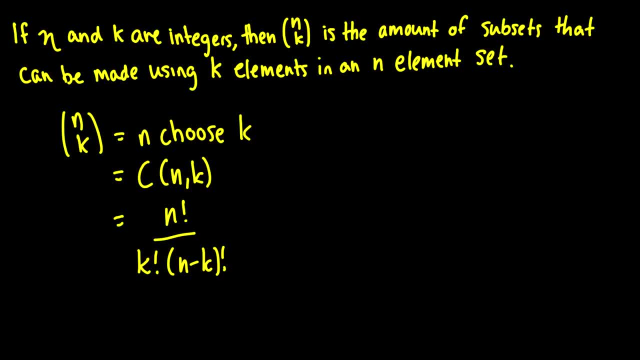 So here's a nice formula for it. If we have two numbers, N and K, then we say that N choose K is the amount of subsets that can be made using K elements in an N element set. So this is written as N choose K. Sometimes you see it as a capital C with N bracket or N comma. 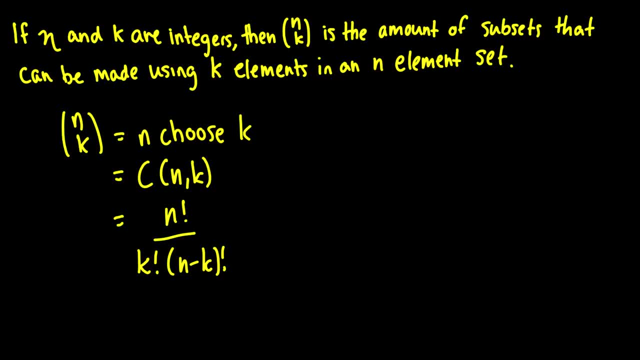 K, just like permutations, And we see the formula here: is N factorial over K factorial, times N minus K factorial, which you'll see is actually just the permutation function divided by K factorial, which is the number of elements we're making. So in the previous 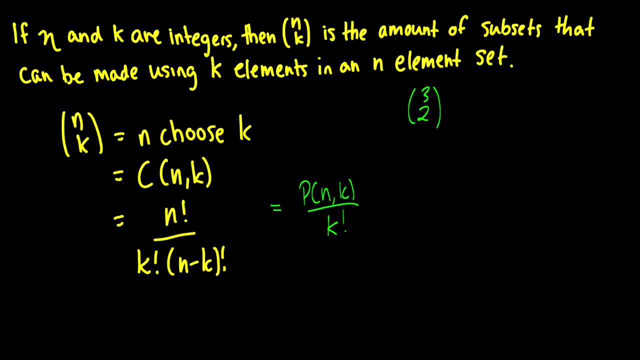 example, you saw three choose two, because we wanted two element combinations out of a three total set. So with this formula, this is going to be three factorial over K factorial is going to be two factorial and N minus K is going to be one factorial, which is going 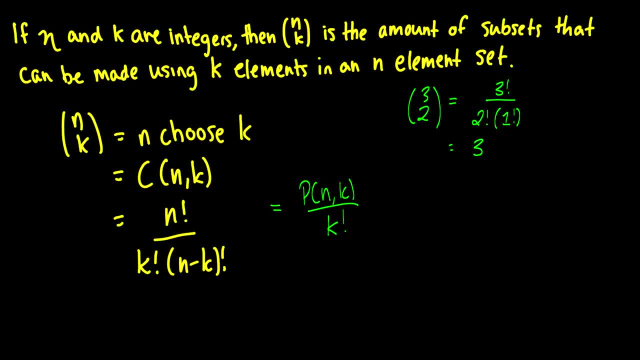 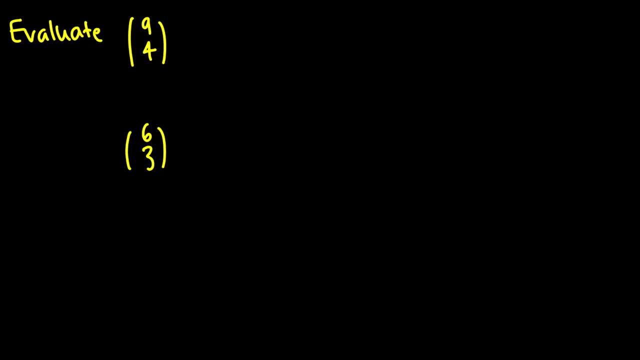 to just be three. So this works. Unfortunately, the amount of permutations there are would also just. the amount of permutations would be six. So there is a bit of a difference there. Anyhow, let's practice with the formula here. So, when we have nine, choose four. we will get. 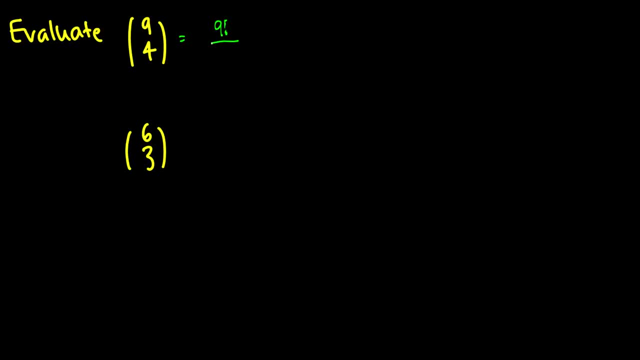 nine factorial on the top, Then we'll get K, which is four factorial times nine minus five, nine minus four, which is five factorial. Essentially, if I were to break it up, it's N? factorial over some number, A factorial plus N factorial over K factorial. So this is going. 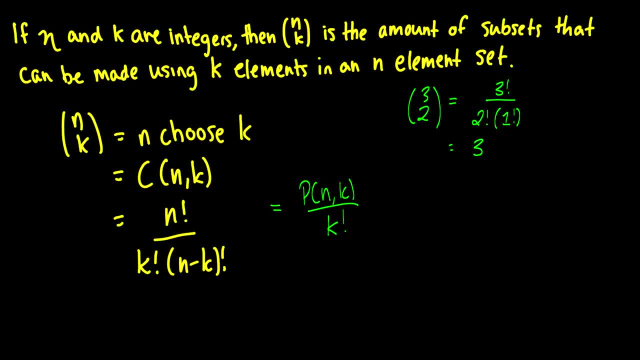 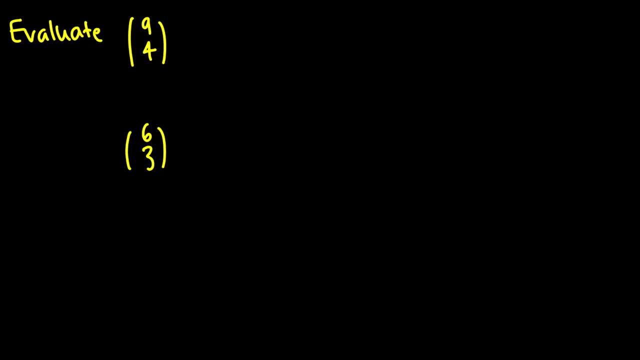 to just be three. So this works. Unfortunately, the amount of permutations there are would also just. the amount of permutations would be six. So there is a bit of a difference there. So let's practice with the formula here. So when we have nine, choose four. we will get. 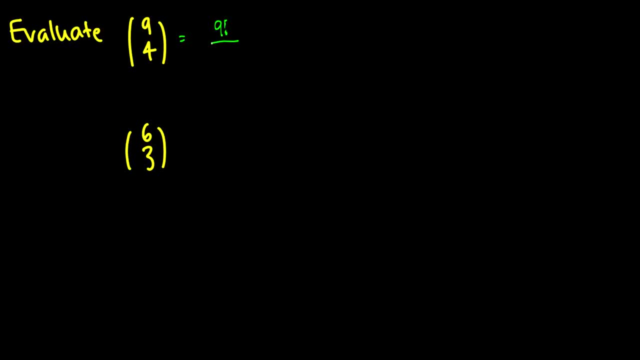 nine factorial on the top, Then we'll get K, which is four factorial times nine minus five, nine minus four, which is five factorial. Essentially, if I were to break it up, it's N factorial over some number, A factorial plus N factorial over K factorial, which is N factorial. 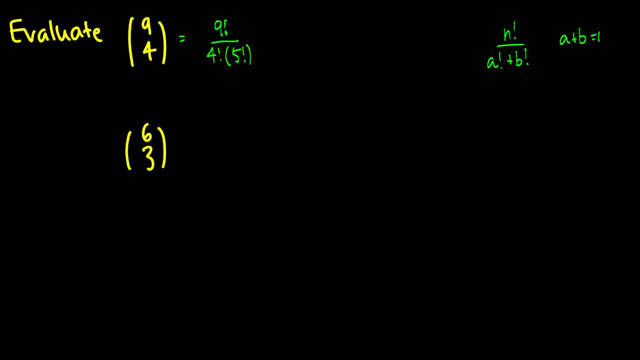 plus B factorial, where A plus B is equal to N. If that makes any sense, I think it should- and it shouldn't be plus. it should be multiplied, But you'll see that the two bottom numbers equal the top number. if you're confused about what the formula is or what, 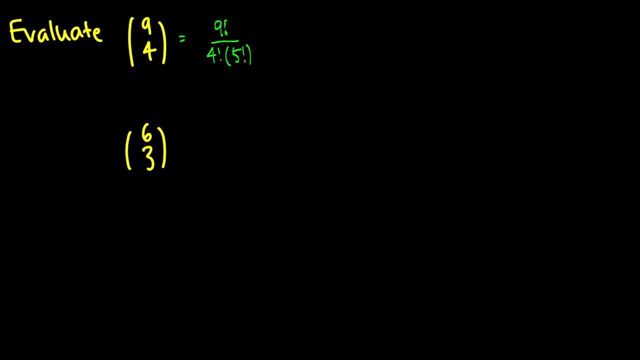 numbers you should be multiplying together as factorials. The two bottom numbers, if you add them, should equal the top. So what we have here is we're going to have nine times eight times seven, Seven times, six times five factorial over four factorial times five factorial You. 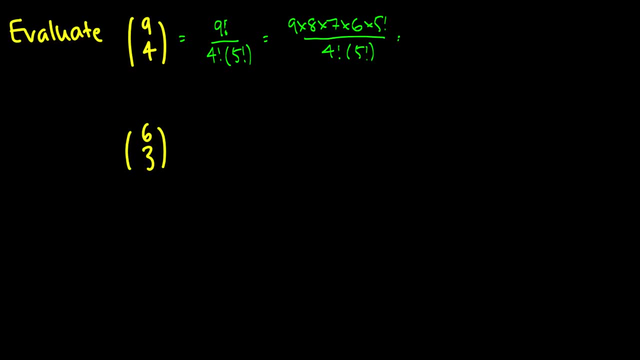 always want to cancel the largest factorial. so that way you're doing the least amount of computational work. So then we're going to get nine times seven times eight times six, over four times, three times, two times one. Now we can simplify things. We see that. 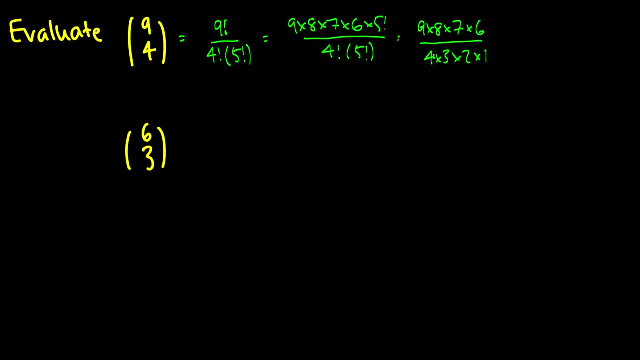 four times two is equal to eight. So we can cancel out the four, the two and the eight, since that's the same thing as eight divided by eight, And we can take the nine and the three and we can simplify this. So we're going to get three times seven times six, which is a little bit more manageable. 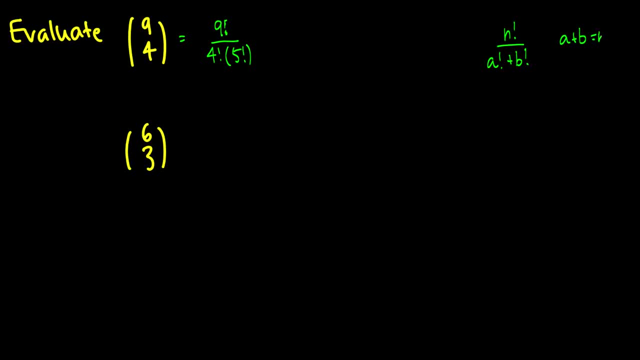 to do this as a personal measurement. Again, this formula is going to have a Civilriers and both doctors comparing it to number one. Nonetheless, we're going to have K factorial over K factorial, plus number two, plus N factorial, which is five factorial over K factorial. If it doesn't make sense, then we're going to have a. 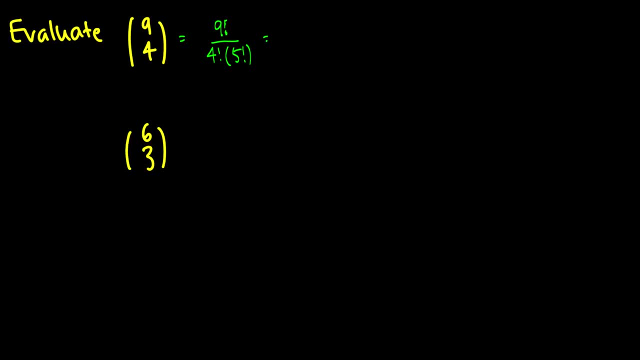 see, yeah, When I do this, we have 9, five factorial over one. Now, that 거죠 the wom 快. So then we have 12 times連 number with plus. Now this delivering is learning the formula, and what we're going to then do here is we're going to do this thing. screw wrong, because 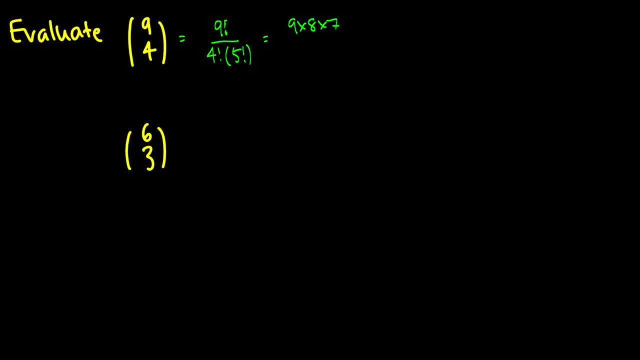 we're going to have nine times n. You can always factor it the other way around. So if you're using here with treasure, ignore 7 times 6 times 5 factorial. over 4 factorial times 5 factorial. You always want to cancel. 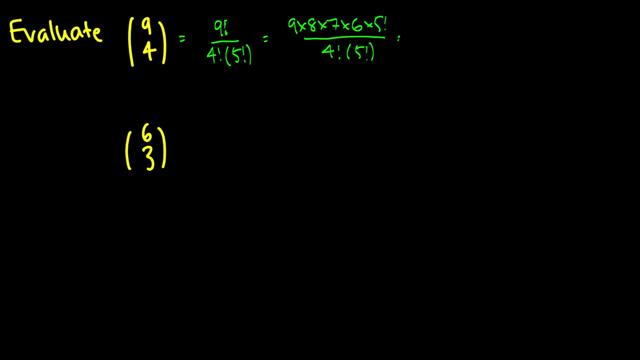 the largest factorial. so that way you're doing the least amount of computational work. So then we're going to get 9 times 7 times 8 times 6 over 4 times 3 times 2 times 1.. Now we can simplify things. We see that 4 times 2 is equal to 8, so we can cancel out the 4,. 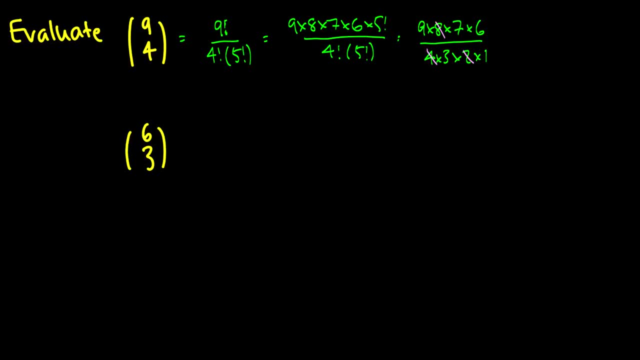 the 2, and the 8,, since that's the same thing as 8 divided by 8.. And we can take the 9 and the 3, and we can simplify this. So we're going to get 3 times 7 times 6,, which is a little bit. 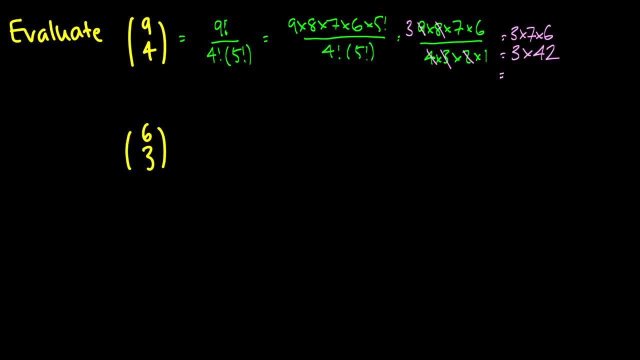 more manageable, because that's 3 times 42, and that's just a hundred And 26.. So 9 choose 4 is 126.. What about 6 choose 3?? Well, this is 6 factorial over 3 factorial times 3 factorial. so this is going to be 6 times 5 times 4.. We're going to cancel one of. 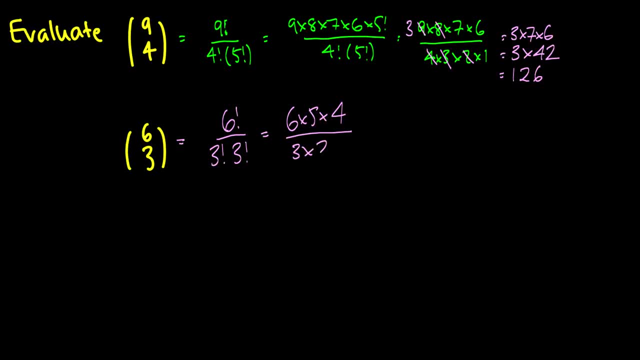 the three factorials on the bottom, then we'll expand the last one. So of course, when we shorten this, we're going to turn the 6 and the 3 into a 2, so I'll have 2 times 6 times 6,. 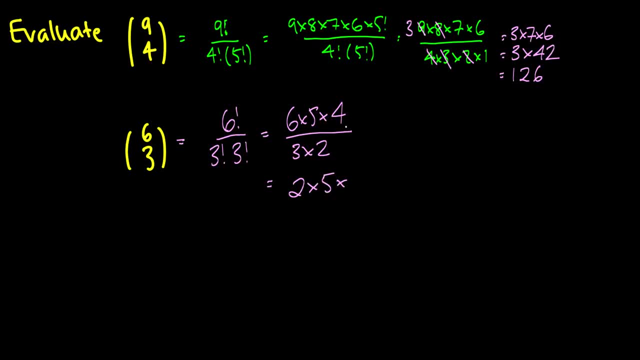 5 times, and then 4 divided by 2 is 2.. So this is going to be 4 times 5,, which is just 20.. Now these calculations will take a bit of practice to get used to. Of course there's 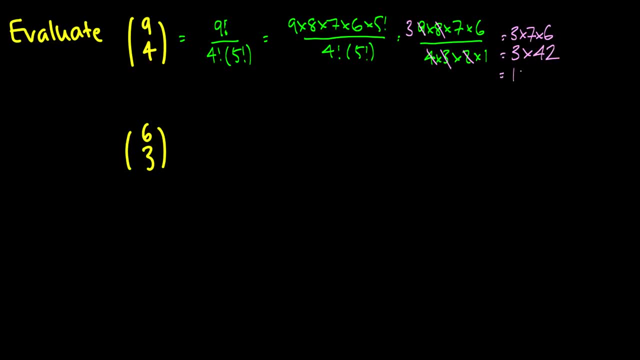 because that's three times forty-two and that's just a hundred and twenty-six. So nine choose four is a hundred and twenty-six. What about six choose three? Well, this is six factorial over three factorial times, three factorial. So this is going to. 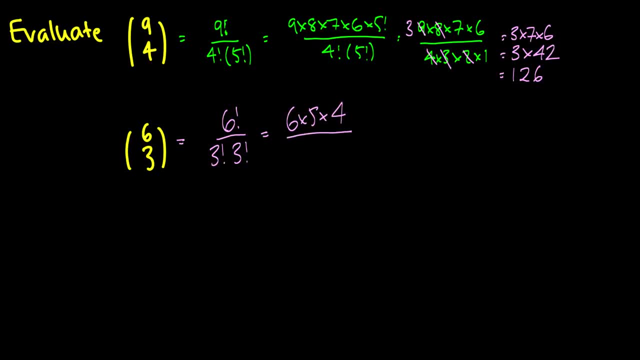 be six times five times four. We're going to cancel one of the three factorials on the bottom. Then we'll expand the last one. So of course, when we shorten this, we're going to turn the six and the three into a two. So two times five times and then four divided. 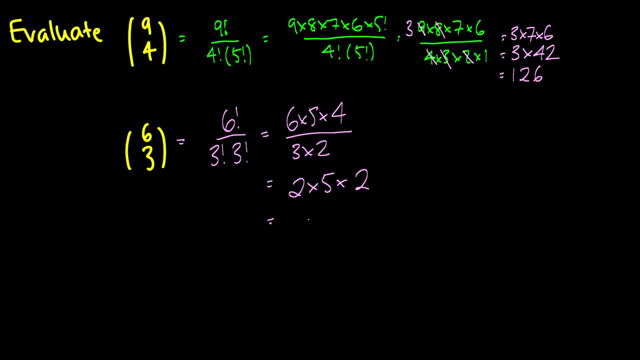 by two is two, So this is going to be four times five. This is going to be four times five, which is just twenty. Now, these calculations will take a bit of practice to get used to. Of course there's a lot of expansions going on, but it's really just a test of your multiplication skills. 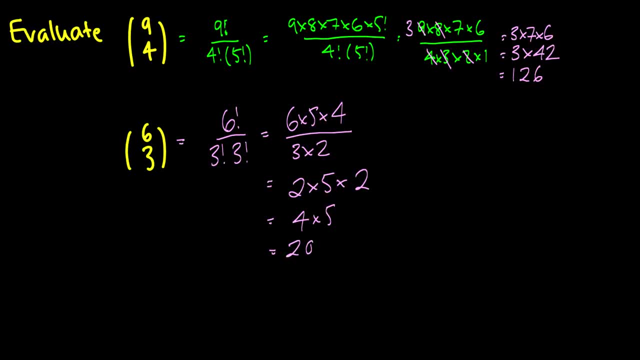 and if you can remember the formula, If you have a calculator graphing calculators, you can even have a function. It's a built-in function that does permutations and combinations, so you just plug in the numbers and it solves it for you. 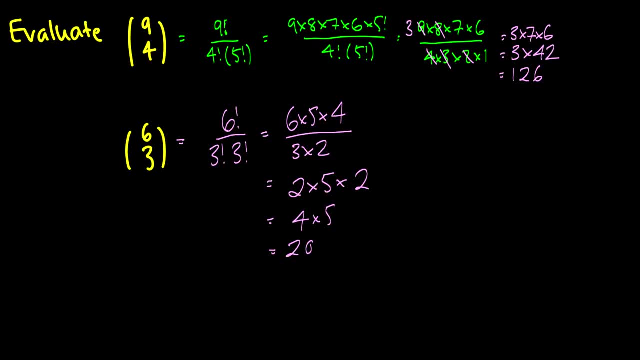 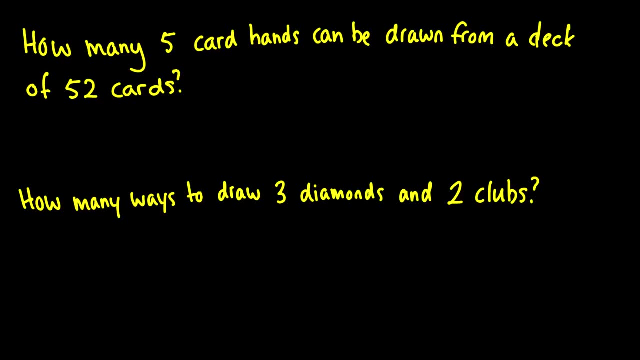 If you have access to that, great, But your questions are going to be pretty much the same, So you're going to have to work probably a little bit harder. Anyways, let's do a couple application questions. How many five-card hands can be drawn from a deck of fifty-two cards? 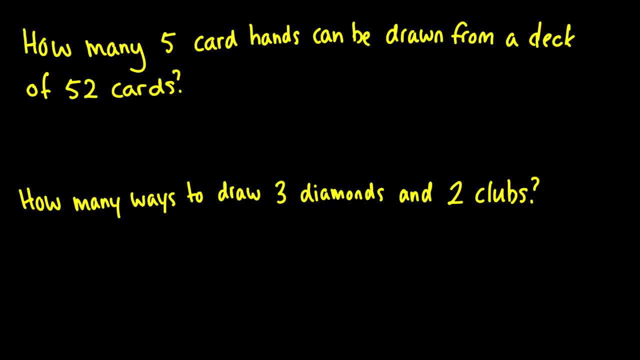 Now your first question is: is this a permutation question or is it a combination question? And you have to know a little bit about cards to know whether or not this is a permutation or combination. When I have five cards in my hand, I can reorder them however I want, and it's never. 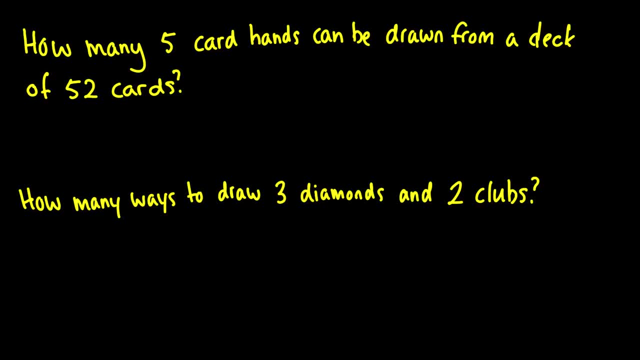 going to change the gameplay. Therefore, this is a combination question. So we have fifty-two total cards and we want to choose five. This is our answer technically. Sometimes you will not have to solve this. Some professors will want you to solve this. 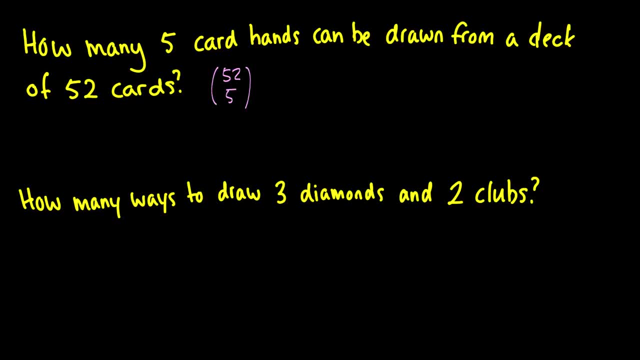 Most on exams will say: do not solve this. leave this as your answer, Which is fine. but for the sake of completion and explaining the formula, I will write this out. So this will be fifty-two factorial over forty-seven factorial times five factorial. 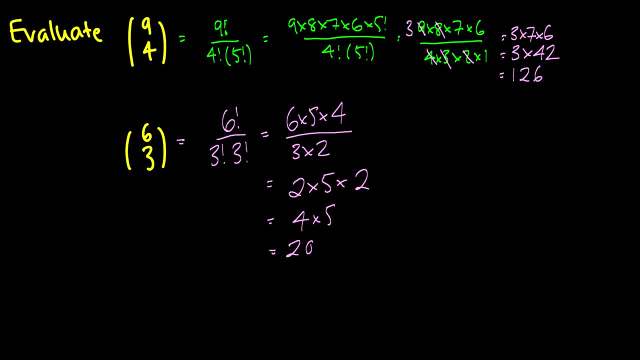 a lot of expansions going on, but it's really just a test of your multiplication skills and if you can remember the formula, If you have a calculator graphing calculators, you can even have a function. It's a built-in function that does permutations and combinations. 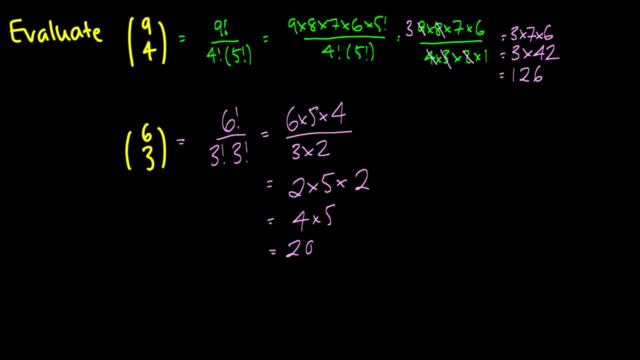 so you can do that. So if you have a calculator, you can even have a function that does permutations and combinations. so you can even have a function that does permutations and combinations. so you just plug in the numbers and it solves it for you. If you have access to that, great. 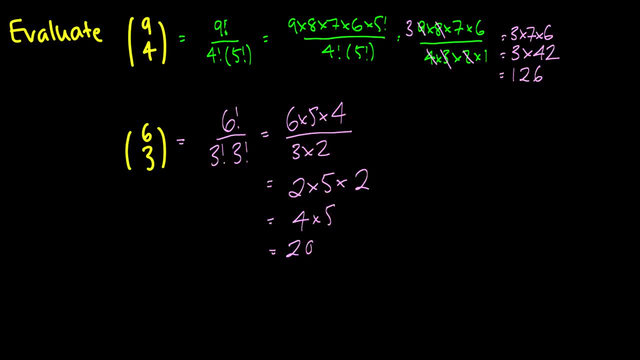 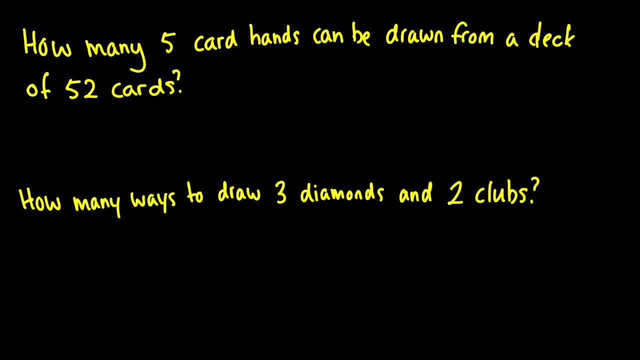 but your questions are going to be probably a little bit harder. Anyways, let's do a couple application questions. How many 5-card hands can be drawn from a deck of 52 cards? Now, your first question is: is this a permutation question or is it a combination question? 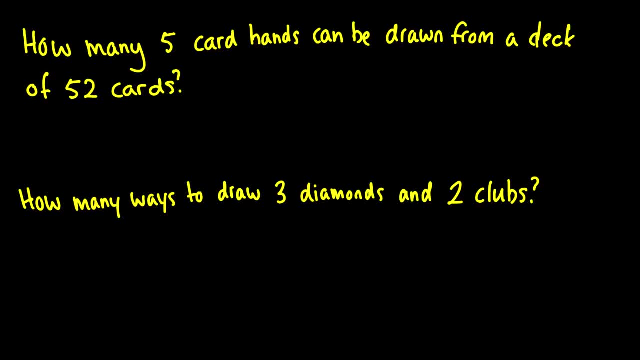 Now your first question is: is this a permutation question or is it a combination question? So you've gotten five cards And you have to know a little bit about cards to know whether or not this is a permutation or combination. When I have five cards in my hand, I can reorder. 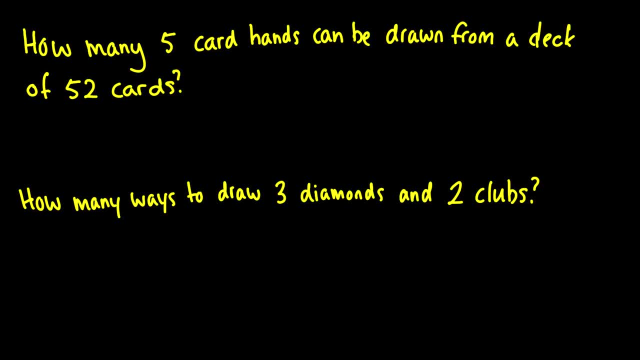 them however I want, and it's never going to change the gameplay. Therefore, this is a combination question. So we have 52 total cards and we want to choose five. This is our answer technically. Sometimes you will not have to solve this, some professors. 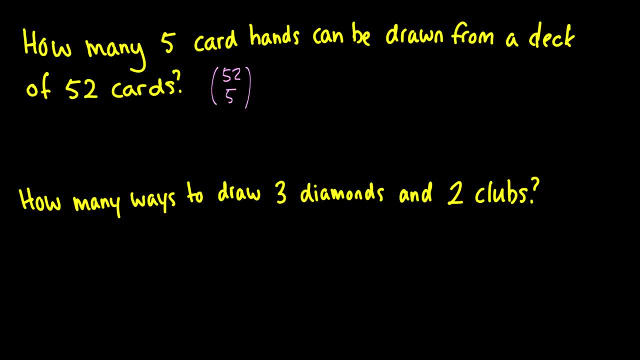 say so Basically, just all of these singles. you don't need to solve this. One or two will want you to solve this. Most on exams will say: do not solve this, leave this as your answer, which is fine, but for the sake of completion and 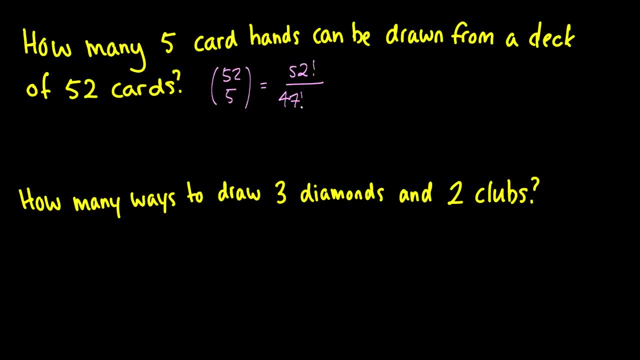 explaining the formula. I will write this out. So this will be 52 factorial over 47 factorial times 5 factorial, which will be 52 times 51 times 50 times 49 times 48, all over 5 times 4 times 3 times 2, and you can see why I didn't. 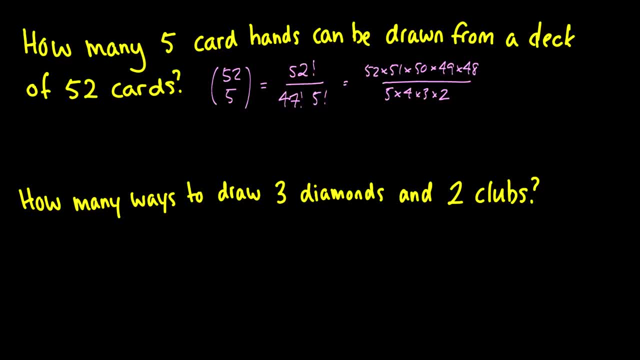 necessarily want to expand this, because this is getting a little bit crazy. However, we can simplify. We can do 2 into 52, so this will be 26 after we simplify the first two. then we can do 51 divided by 3 is. 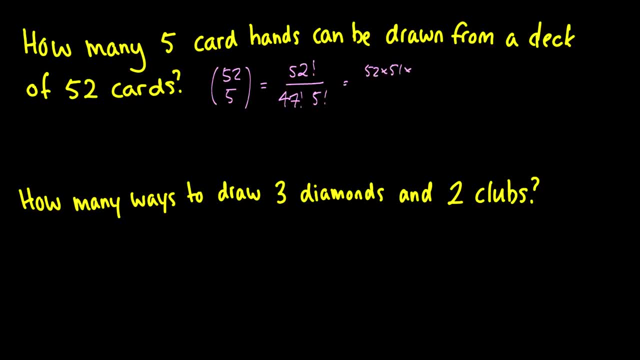 which will be fifty-two times fifty-one times fifty times forty-nine times forty-eight, all over five times four times three times two. You can see why I didn't necessarily want to expand this, because this is getting a little bit crazy. However, we can simplify. We can do two into fifty-two, so this will. 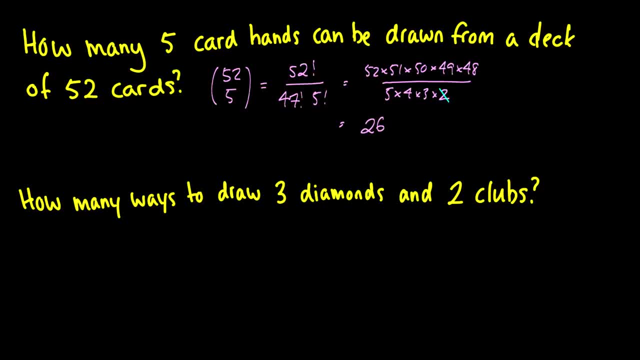 be twenty-six after we simplify the first two. Then we can do: fifty-one divided by three is seventeen. fifty divided by five is ten. forty-eight divided by four is twelve, and then we have this ridiculous forty-nine. Now, of course, I still do not want to do this by hand, so we will leave the answer. 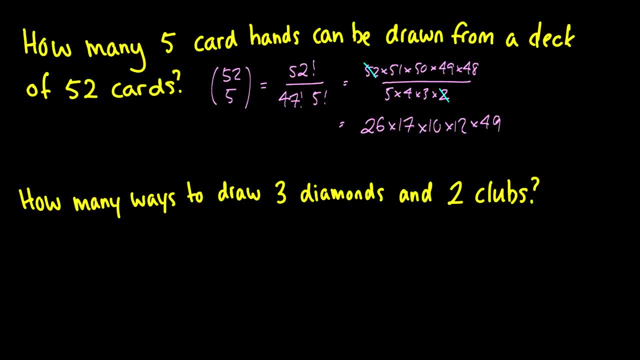 like that. That is basically the best you can simplify it without a calculator, unless you are really really crazy and want to somehow figure out what four hundred and ninety times twelve is. then multiply that by seventeen, then twenty-six. I do not think anyone wants. 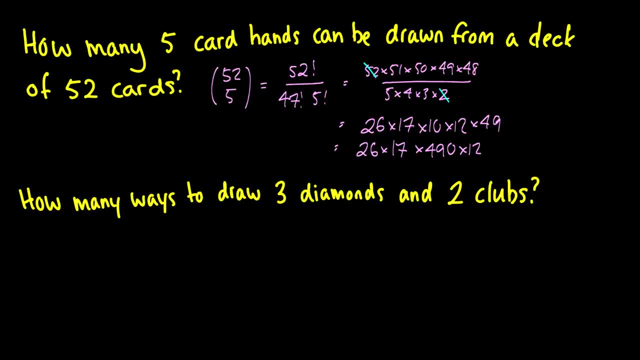 to do that. We will leave it at that. Now here is a better question: How many ways can we draw three-diamonds? Well, this is a little bit more interesting, because when we just draw five cards, we can do it really however we want. We just say, oh, there are fifty-two total cards, and then 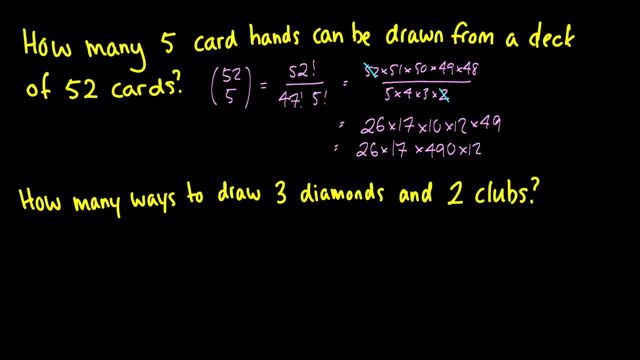 we draw five and it is not too bad. However, there are a couple of things we need to know. First of all is how many diamonds are there in the deck And what is the number of clubs in the deck? Well, there are thirteen of each suit, so there are going to be thirteen diamonds and 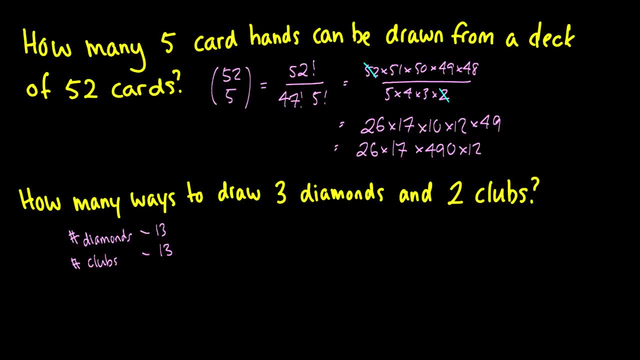 thirteen clubs and we just want to draw three diamonds and two clubs, and it does not matter what order we draw them in. So we say, okay, three diamonds, that means we have thirteen ones we can choose from, and we just want to choose three. 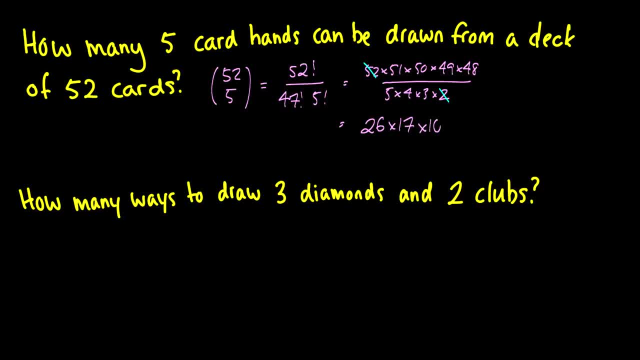 17,. 50 divided by 5 is 10,, 48 divided by 4 is 12,, and then we have this ridiculous 49.. Now, of course, I still don't want to do this by hand, so we'll leave the. 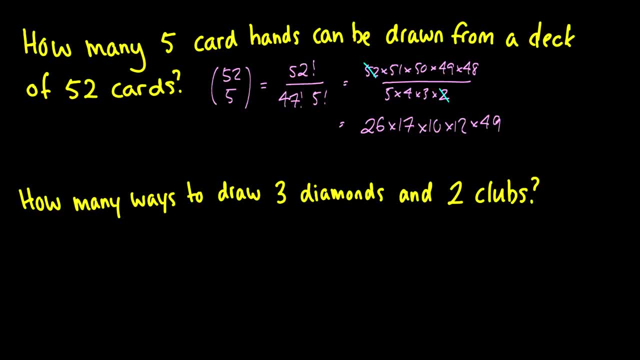 answer like that, and that's basically the the best. you can simplify it without a calculator, unless you're really, really crazy and want to somehow figure out what 490 times 12 is. then multiply that by 17,, then 26.. So I don't think anyone wants to do that. we'll leave it at that. 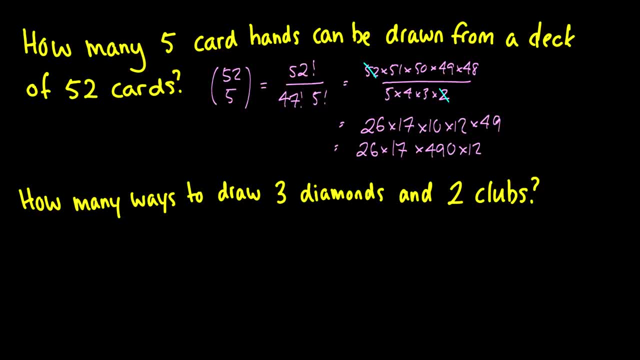 Now here's a better question: How many ways can we draw three diamonds and two clubs? Well, this is a little bit more interesting, because when we just draw five cards, we can do it really however we want. We just say, oh, there's 52 total. 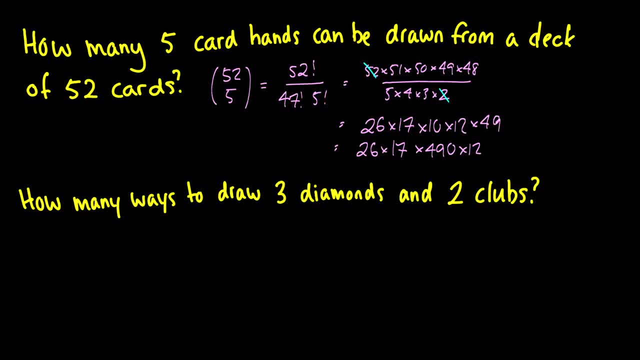 cards and then we draw five, and it's not too bad. However, there are a couple things we need to know. First of all is how many diamonds are there in the deck and what is the number of clubs in the deck? Well, there's 13 of. 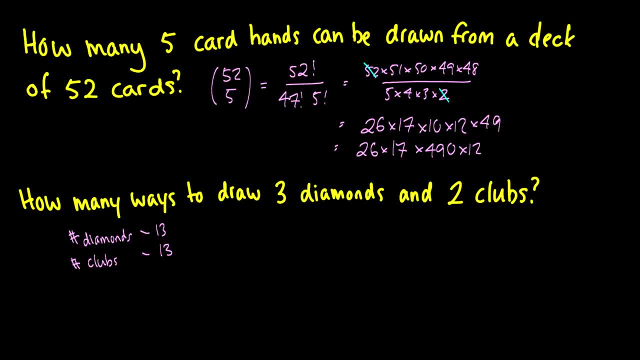 each suit. so there's going to be 13 diamonds and 13 clubs and we just want to draw three diamonds and two clubs, and it doesn't matter what order we draw them in. So we say, okay, three diamonds, that means we have 13 ones. we 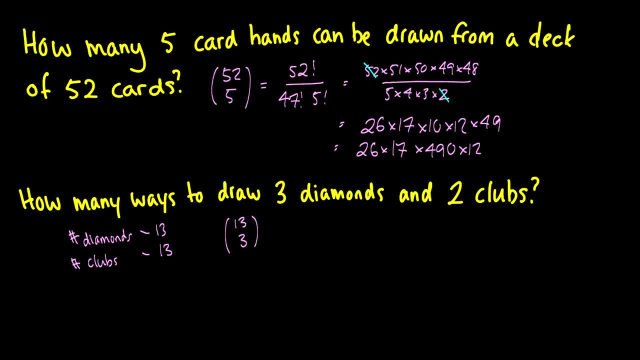 can choose from, and we just want to choose three. So this is the diamonds, and then we multiply that by the 13, choose two clubs, and this will get you your answer. So basically, your answer is going to be 13. choose three times 13: choose. 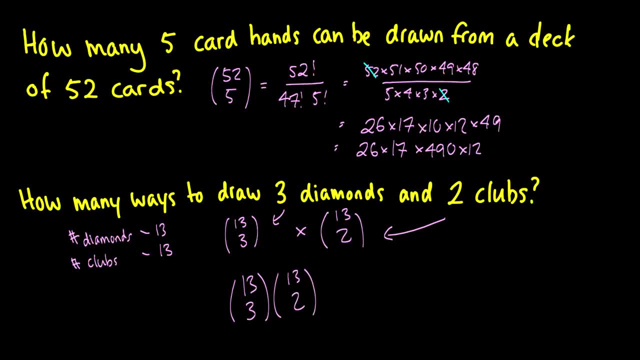 two, and I'm going to mention right off the bat: this is not the same as 13 choose four. that is not the same. this is not how combination multiplication works, so do not make this mistake. there is a very interesting way, which I'm going to show. 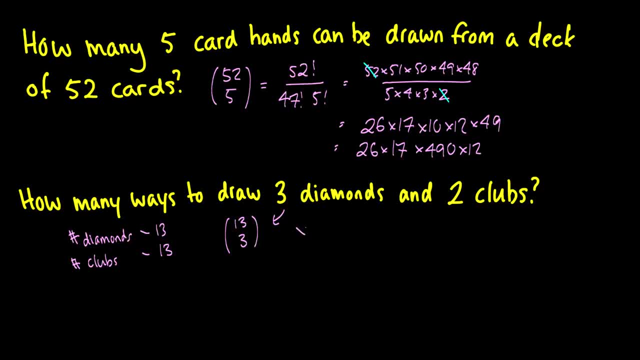 So this is the diamonds, And then we multiply that by the thirteen: choose two clubs, And this will get you your answer. So, basically, your answer is going to be: thirteen, choose three times thirteen, choose two. And I am going to mention right off the bat this is not the same as thirteen choose five. 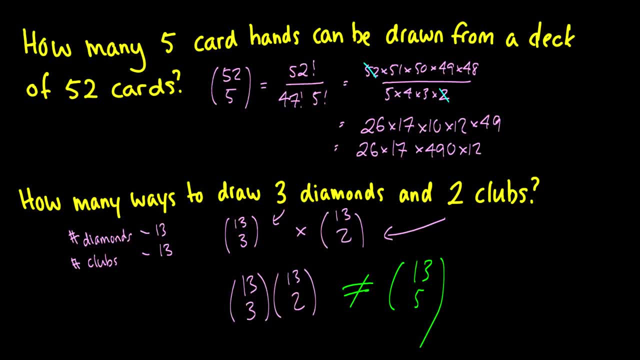 That is not the same. This is not how combination multiplication works, So do not make this mistake. There is a very interesting way, which I am going to show you in a second, how we can do addition with combinations. But that is about as far as you can go without proving some really weird and difficult theorems. 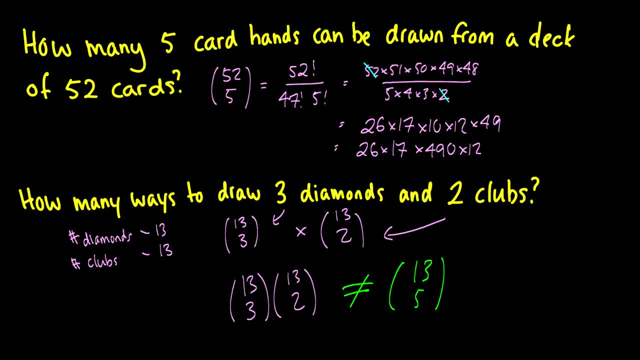 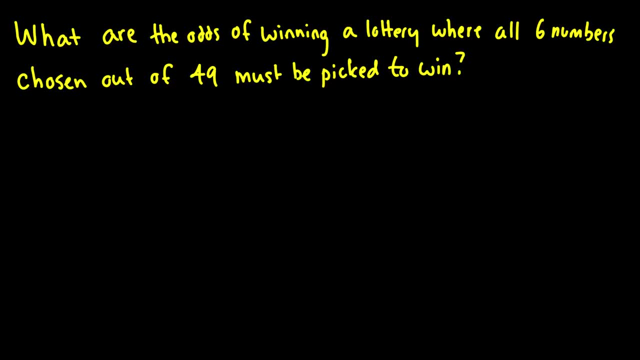 which hopefully you will get to do in your course. But first one more question: What are the odds of winning a lottery where all six numbers should be equal to one? What are the odds of winning a lottery where all six numbers should be equal to one? 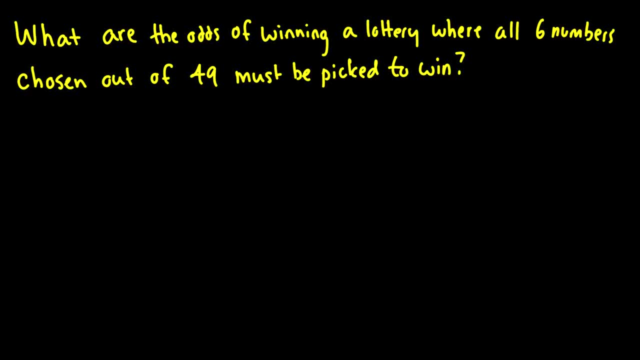 What are the odds of winning a lottery where all six numbers should be equal to one, A lottery where all six numbers chosen out of forty-nine must be picked to win? Now, this is a little bit different, because I am asking for the odds, And when I say the odds I mean the situation that it occurs in. 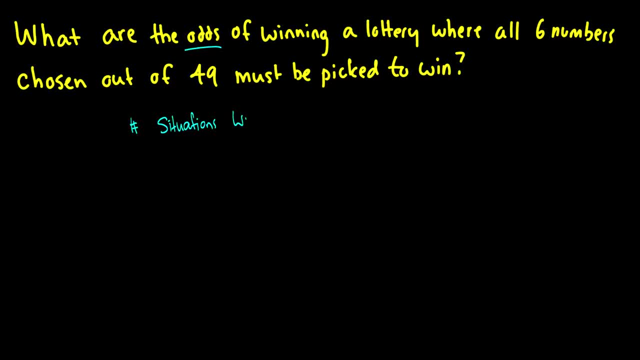 So the number of situations where you win divided by the number of total situations, Okay. so what's interesting is that if we can only pick six numbers and all of them have to be chosen, then there's only going to be one situation where we can win. 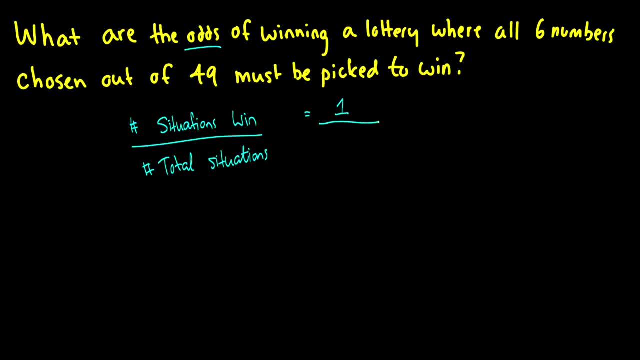 But how many total ways are there to do this? Well, we just have to choose six numbers out of 49. So we're going to have 49, choose 6 on the bottom. And this is your answer. And you have to be very careful because we talk about the odds. 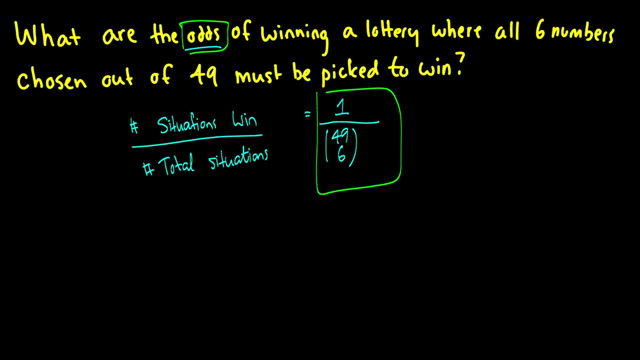 So it's the number of ways you can win over the number of total situations you can do it. So we have 1 over 49. choose 6, because of course there's 49 numbers in the lottery and you have to pick 6.. 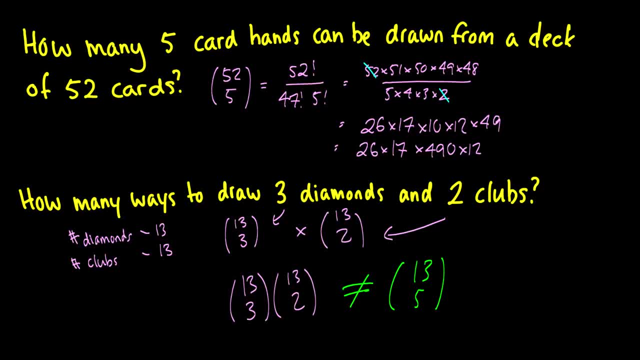 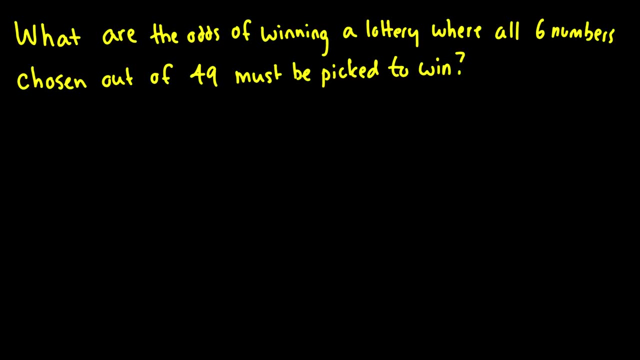 you in a second how we can do addition with combinations. but that's about as far as you can go without proving some really weird and difficult theorems which hopefully you'll get to do in your course. but first one more question: what are the odds of winning a lottery where all six 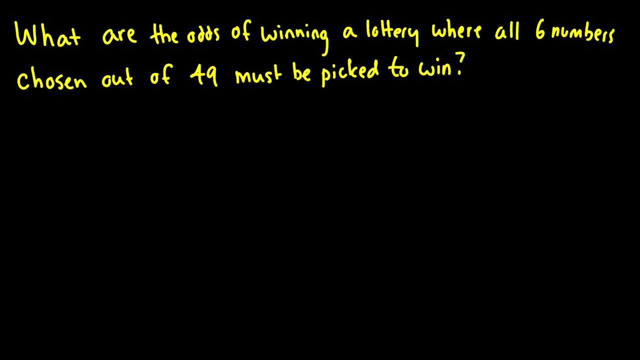 numbers chosen out of 49 must be picked to win. now this is a little bit different, because I'm asking for the odds, and when I say the odds, I mean the, the situation that it occurs in. so the number of situations where you win divided by the number of total situations. okay, so what's interesting is that if we we 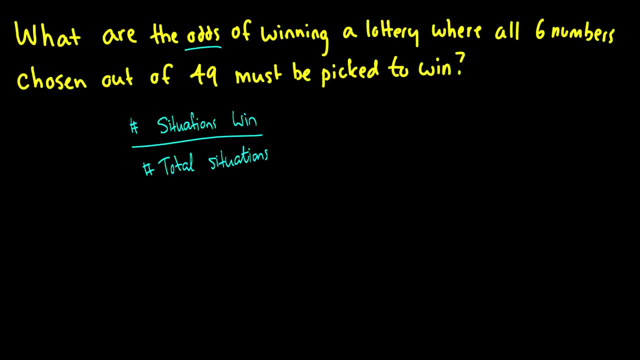 can only pick six numbers and all of them have to be chosen, then there's only going to be one situation where we can win. but how many total ways are there to do this? well, we just have to choose six numbers out of 49. so we're gonna have 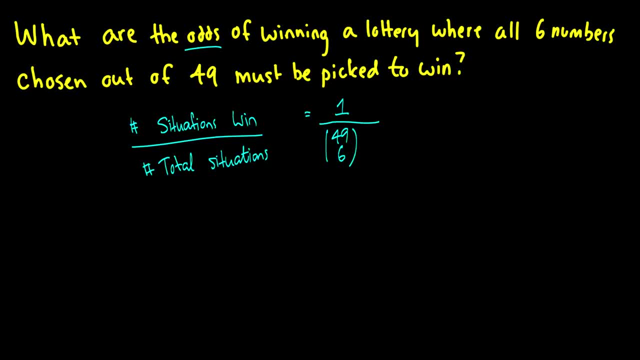 49. choose six on the bottom and this is your answer. and you have to be very careful because we talked about the odds, so it's the number of ways you can win over the number of total situations you can do it. so we have one over 49 choose. 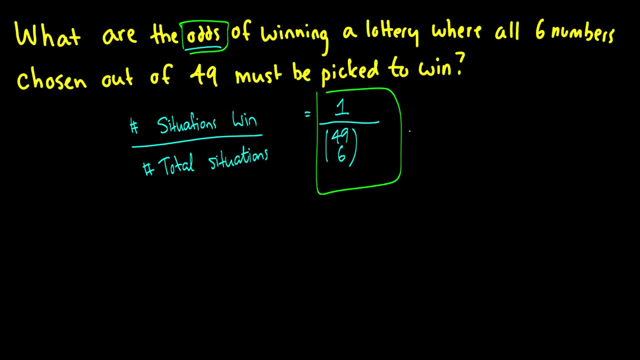 six, because of course there's 49 numbers in the lottery and you have to pick six numbers. and you have to pick six numbers. and you have to pick six numbers, pick six. and if you know anything about lottery tickets, when you have your ticket here it'll say something like lotto max at the top and it'll list your 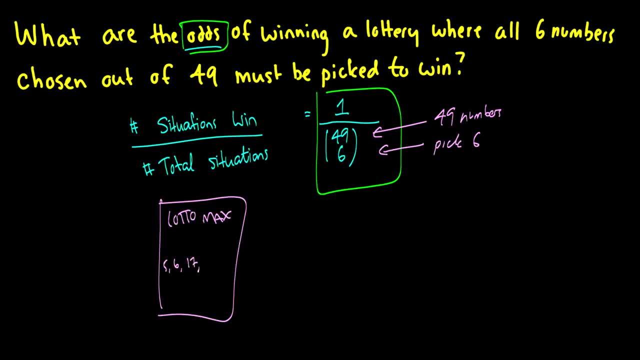 numbers in chronological order at the bottom here. so the order doesn't matter, because it's going to be listed chronologically anyway. if the permutation had to be perfect, there would be a lot less winners. in fact, in this scenario, if the permutation mattered, there would be six factorial. well, your chance would. 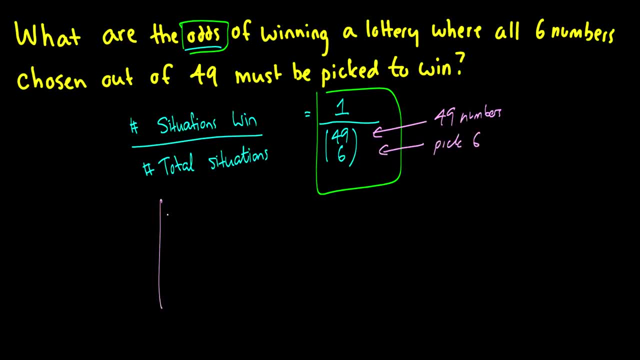 And if you know anything about lottery tickets, when you have your ticket here it'll say something like Lotto Max at the top And it'll list your numbers in chronological order at the bottom here. So the order doesn't matter, because it's going to be listed chronologically anyway. 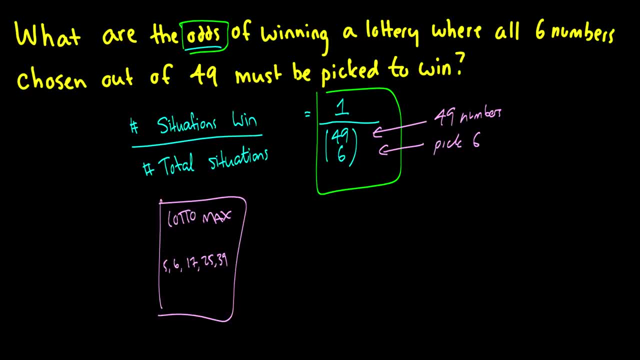 If the permutation had to be perfect, there would be a lot less winners. In fact, in this scenario, if the permutation mattered, there would be 6 factorial well, your chance would decrease, Or, yeah, your chance would decrease. 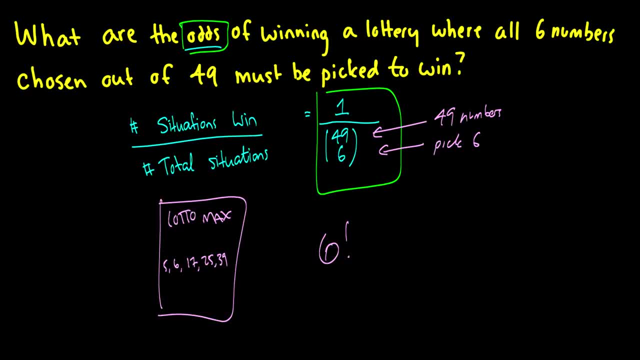 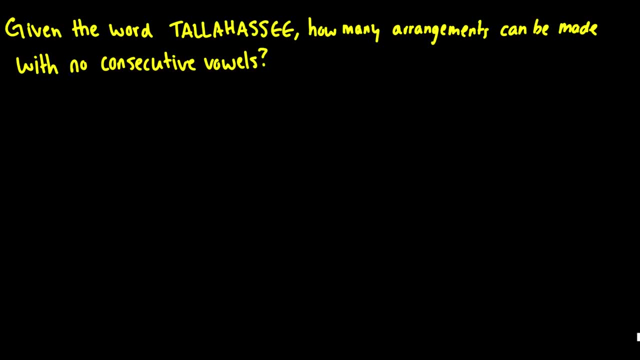 But it's going to be 6 factorial. It's going to decrease by a magnitude of 6 factorial if this were the case, where permutation was important. Now, given the word Tallahassee. so this is a little bit interesting because we're going. 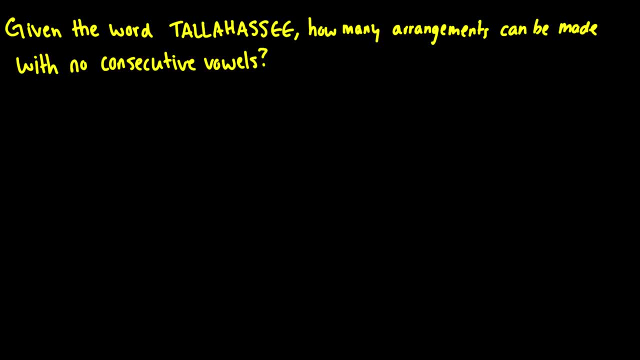 to combine something we learned in permutations and combinations: How many ways or how many arrangements can be made with this word where there's no consecutive vowels? This is an interesting problem. So we're going to do what we did before And we're going to list all the letters out. 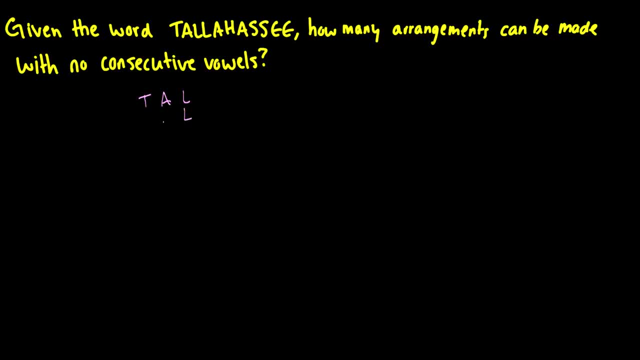 We're going to stack them, so we know how many of each letter there are- Tallahassee. So, okay, we have 3 A's, 2 L's, 2 S's and 2 E's. Of course we have lots of these, otherwise I wouldn't have picked this question. 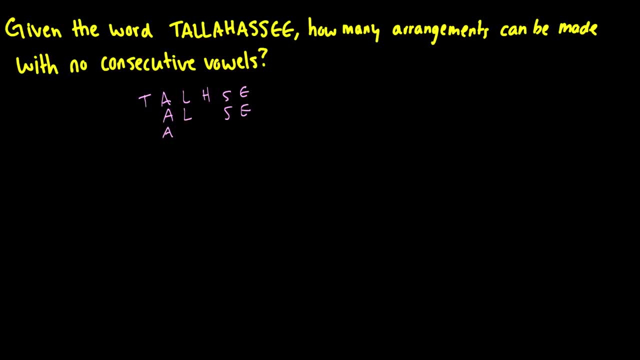 Now how many arrangements can be made with no consecutive vowels? So a strategy here is saying: Let's leave the vowels out for now. Let's look at those later. So now we have a word that is T, L, L, H, S, S, And we ask ourselves: how many ways can we arrange this word? 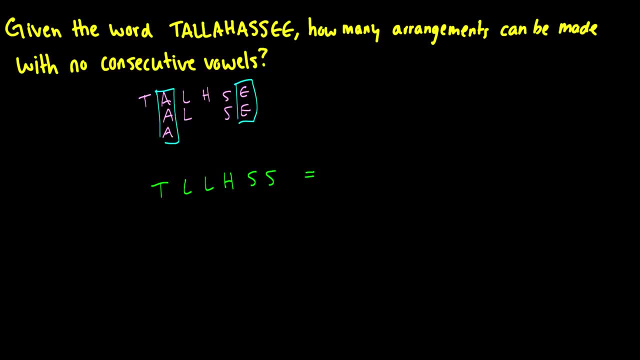 Well, this should be fairly simple. We see there's 6 total letters, so that's 6 factorial. We have 2 L's, so we divide by 2 factorial. We have 2 S's, So we divide by 2 factorial. 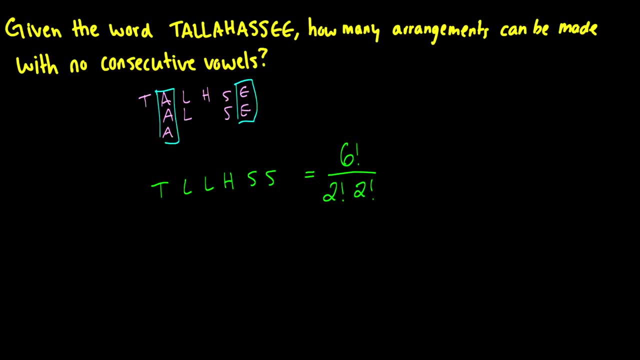 We have 2 factorial because they are indistinguishable from each other. So here's the first part. We're going to have to multiply this by something, But how do we figure out what to do with the vowels here? Well, remember that order does not matter. 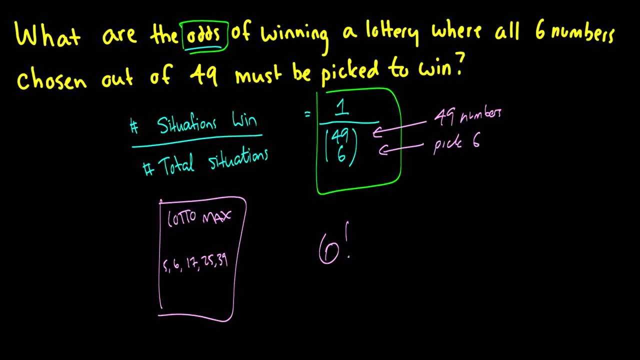 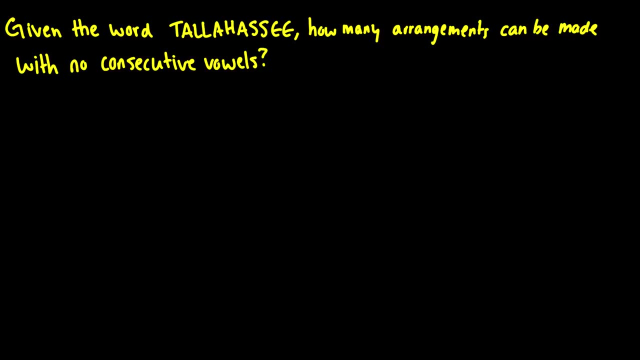 decrease, or your chance would decrease by a magnitude of six factorial if this were the case where permutation was important. now, given the word Tallahassee. so this is a little bit interesting because we're going to combine something we learned in permutations and combinations: how many ways or how many arrangements can be made with this word where there's. 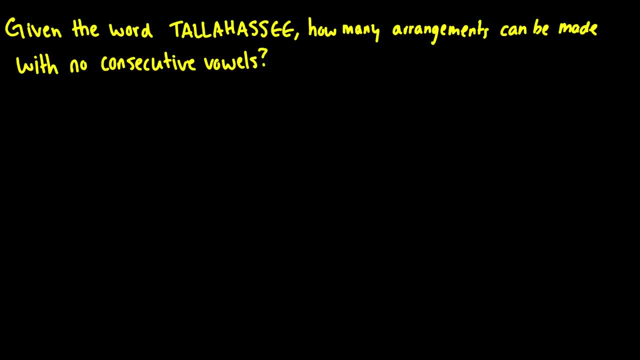 no consecutive vowels. this is an interesting problem. so we're going to do what we did before and we're going to list all the letters out. we're gonna stack them so we know how many of each letter there are: Tallahassee. so okay, we have three a, two L's, two S and two E's. of course, 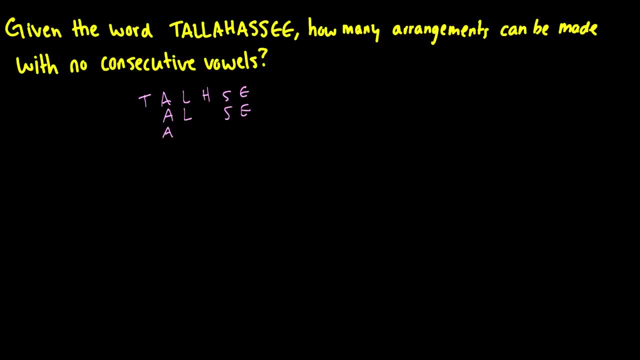 we have lots of these, otherwise I wouldn't have picked this question Now. how many arrangements can be made with no consecutive vowels? So a strategy here is saying: let's leave the vowels out for now. Let's look at those later. So now we have a word that is T-L-L-H-S-S. 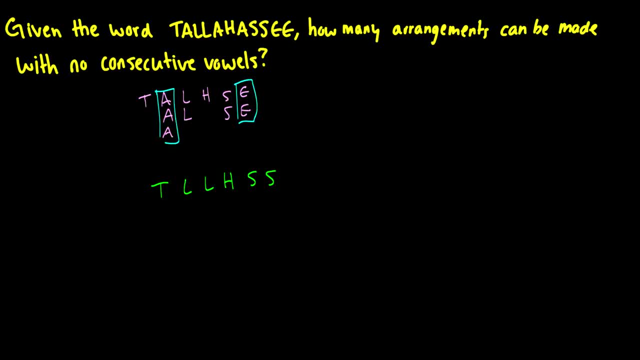 and we ask ourselves: how many ways can we arrange this word? Well, this should be fairly simple. we see there's six total letters, that's six factorial. we have two L's, so we divide by two factorial. we have two S's, so we divide by two factorial, because they are indistinguishable from. 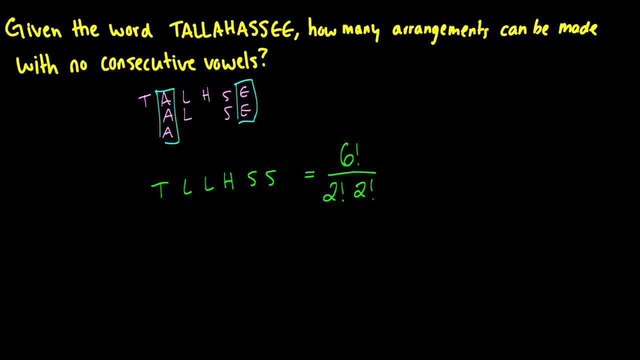 each other. So here's the first part. We're going to have to multiply this by something, but how do we figure out what to do with the vowels here? Well, remember that order does not matter. So where can we place the vowels here? We can place one before the T, between the T and the L. 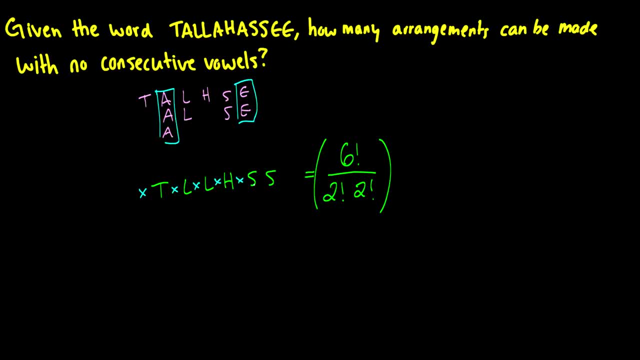 between the L and the L, L and the H, H-S, S-S and right after the S. So there's one, two, three, four, five, six. there's seven positions we can choose to put the vowels, So that's seven. 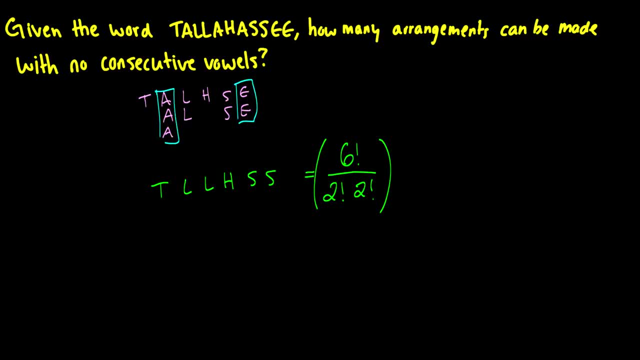 So where can we place the vowels here? We can place one before the T, Between the T and the L, between the L and the L, L and the H, H, S, S, S and right after the S. So there's 1,, 2,, 3,, 4,, 5,, 6, there's 7 positions we can choose to put the vowels. 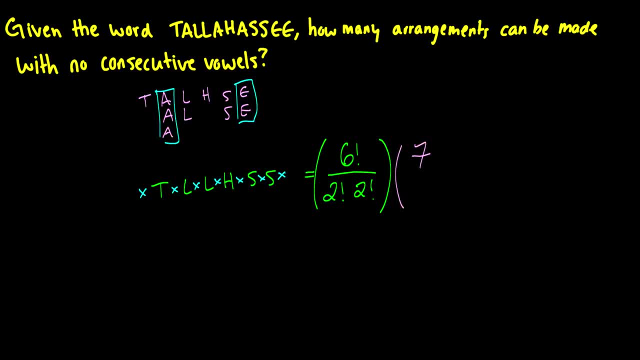 So that's 7.. And there's 5 vowels, so we have to choose 5.. Okay, so now we've chosen 5 out of 7 positions. Now there's still one more step to the puzzle, And now we have A, A, A, E, E. Well, we still have to order these ones too, because there's 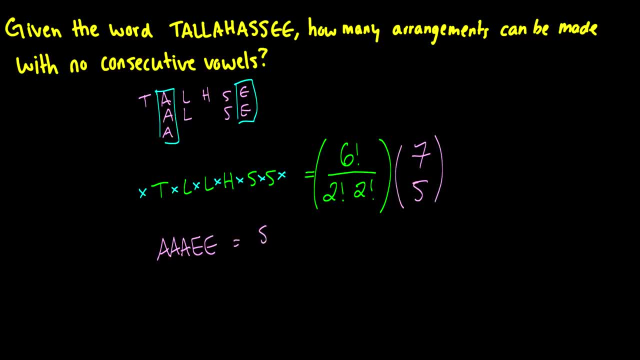 different arrangements. So there's going to be 5 factorial of these vowels over 3 factorial times 2 factorial. So we then have to multiply it by 5 factorial over 3 factorial by 2 factorial. So this question got really messy. 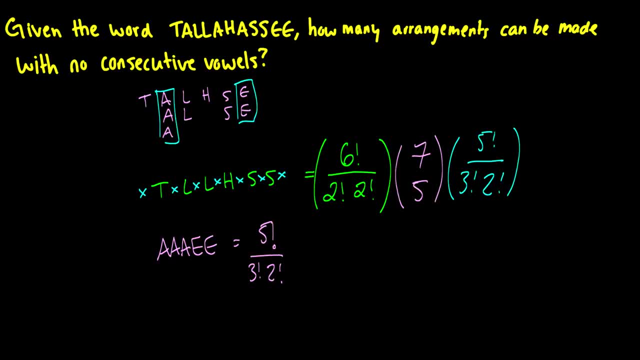 And conceptually It seems like a very easy problem And it sort of is, but wondering: oh, where do I start to break it down? Where do I go next? This is the difficult part. So when you say, okay, I don't want this group of things to be together, you separate them. 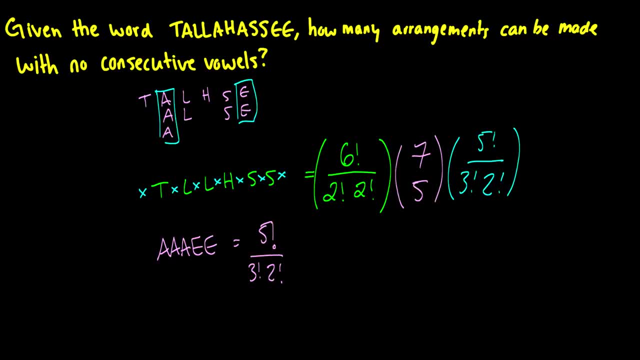 from the group. you figure out the number of arrangements of the rest of the things, you figure out the number of arrangements of the things you're trying to keep separate and then you just see how many spots you can put those other things into them. 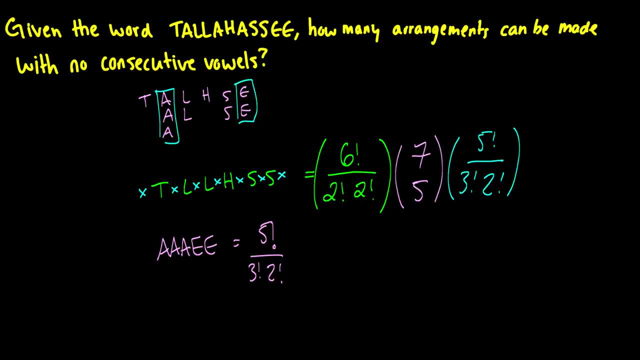 And then you choose the amount that you need. So in this case we listed out all the letters. We said, okay, we want the vowels separated, So let's figure out how many ways we can sort the consonants. Let's see the amount of spaces we have for the vowels to put into after we have arranged. 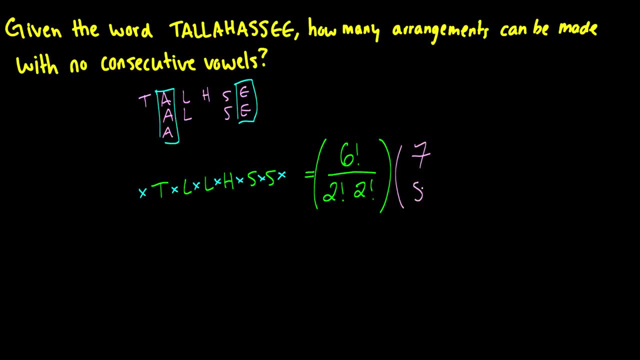 and there's five. Okay, so now we've chosen five out of seven positions. Now there's still one more step to the puzzle, and now we have A-A-A-E-E. Well, we still have to order these ones too, because 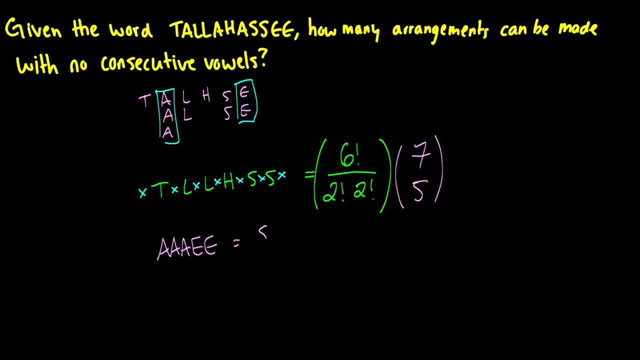 there's different arrangements. So there's going to be five factorial of these vowels over three factorial times two factorial. so we then have to multiply by two factorial and we have to multiply it by five factorial over three factorial, by two factorial. So this question got really. 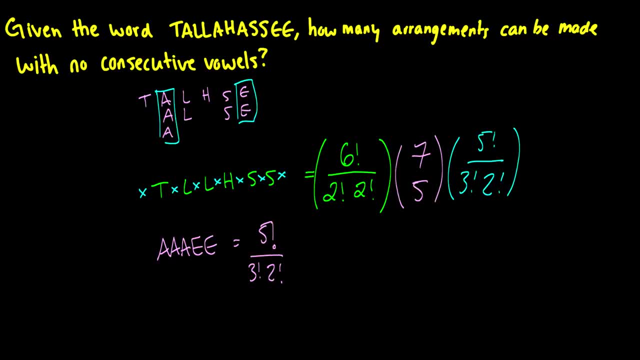 messy and conceptually it seems like a very easy problem- and it sort of is- but wondering, oh, where do I start to break it down? Where do I go next? This is the difficult part. So when you say, okay, I don't want this group of things to be together, 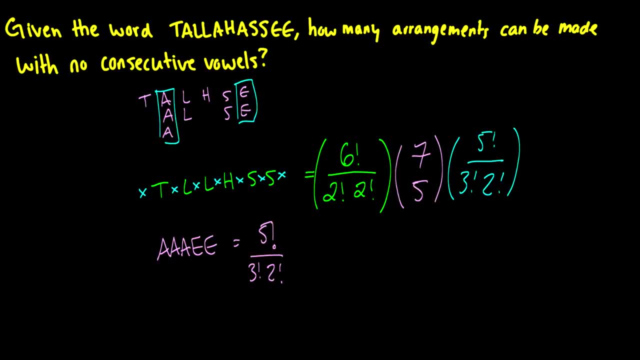 you separate them from the group. you figure out the number of arrangements of the rest of the things you're trying to keep separate, and then you just see how many spots you can put those other things into them and then you choose the amount that you need. So in this case we listed out all. 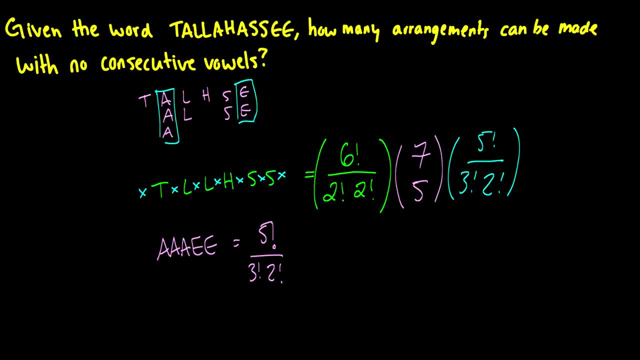 the letters. We said, okay, we want the vowels separated. so let's figure out how many ways we can assort the consonants. Let's see the amount of spaces we have for the vowels to put into after we have arranged our consonants. 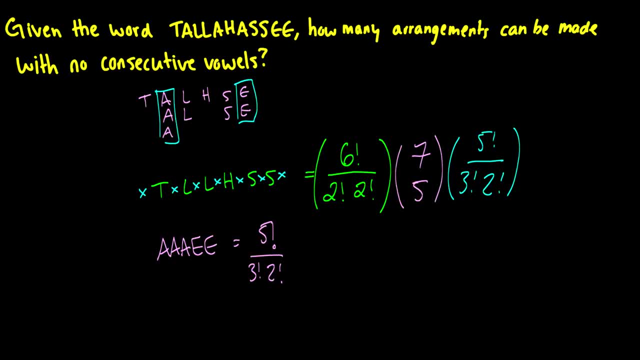 and then how many ways can we arrange those vowels before we put them into the different positions? So, anyways, that was some introduction to combinations. We get to see some cool things we can do with combinations and how they relate to this very cool structure called Pascal's. 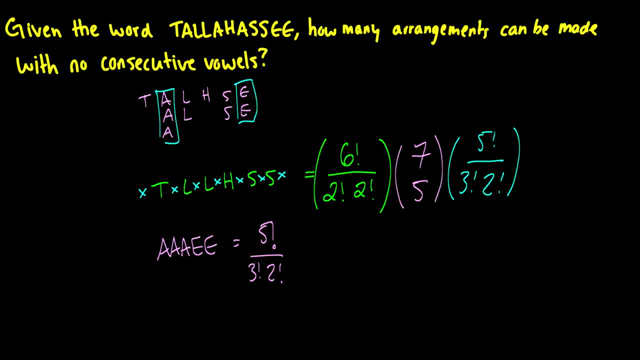 Triangle in the following video, which I think is a lot cooler than this stuff here. if you find mathematics and combinations cool- which I hope- if you're watching a video 17 minutes in on YouTube on your spare time, you do find mathematics a little bit cool. 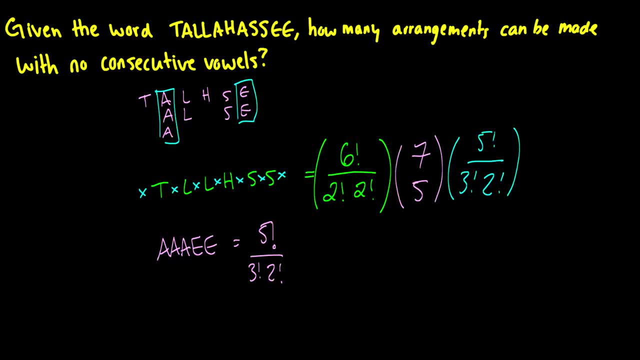 If not, I don't know why you're taking the course or why you're watching it, but I mean, if it's for me and you love my voice, thanks a lot. but you're kind of weird, I'm just kidding. 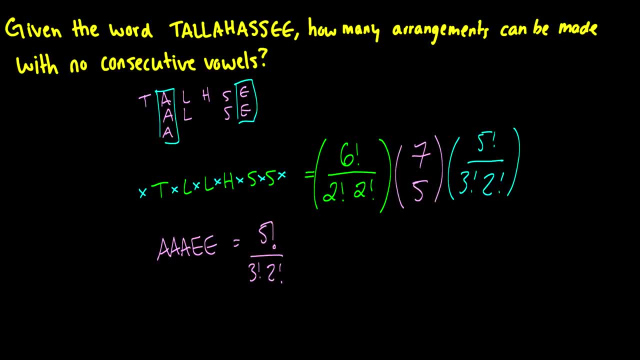 Anyways, if you have any questions, as always, leave them in the comments and I'll get to them as quickly as I can.